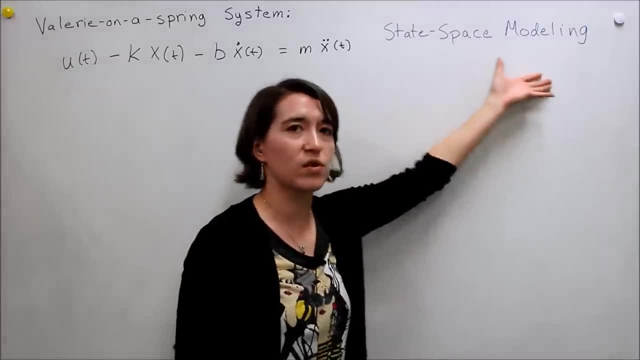 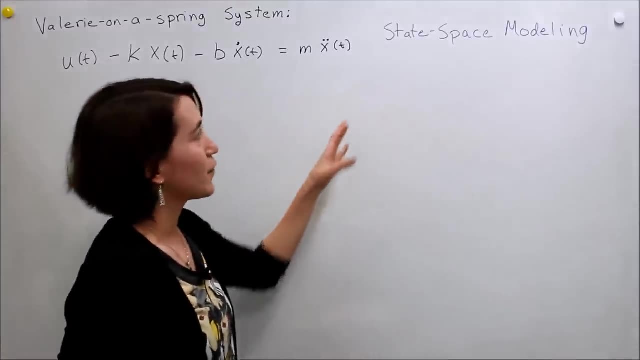 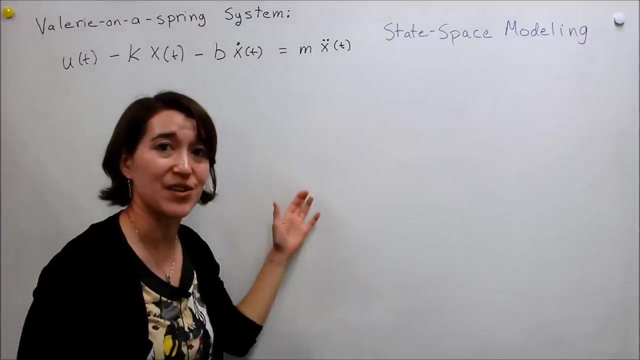 multiple outputs. So this is more used for complex systems and it's a very powerful modeling tool. So we're going to talk about that And first we're going to go back to an example that I hope you remember: the Valerie-Honest-Spring system, where Valerie was attached. 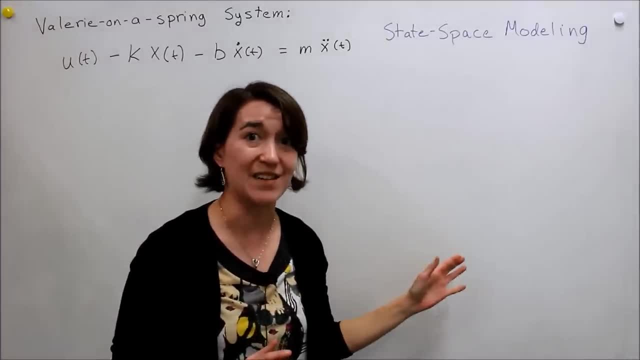 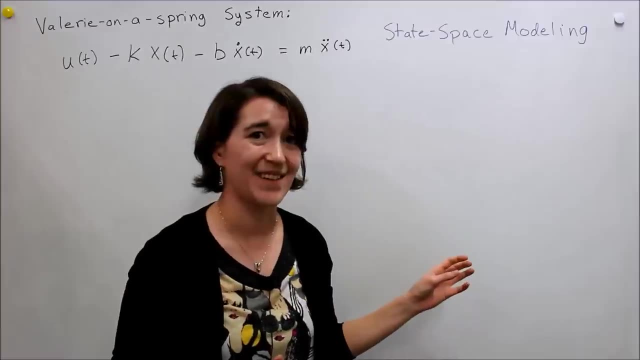 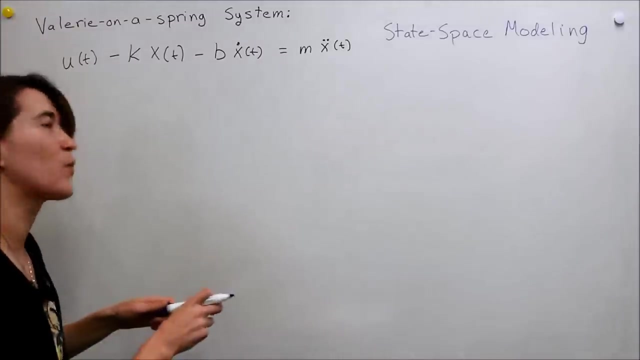 to an unmovable box of green tea. So if you don't remember that here, it is OK. so you remember the system, Great. So here is the equation that we derived last time, and let's just remember what these things mean. This was the input force that we were putting onto. 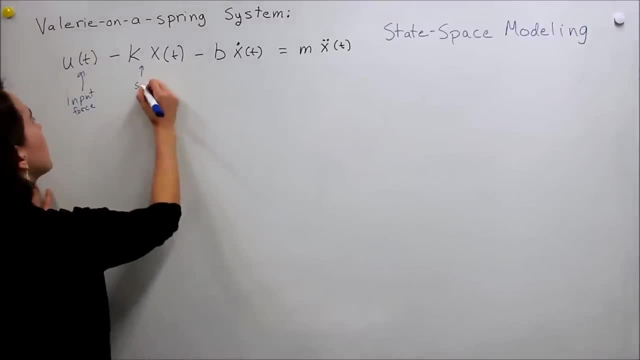 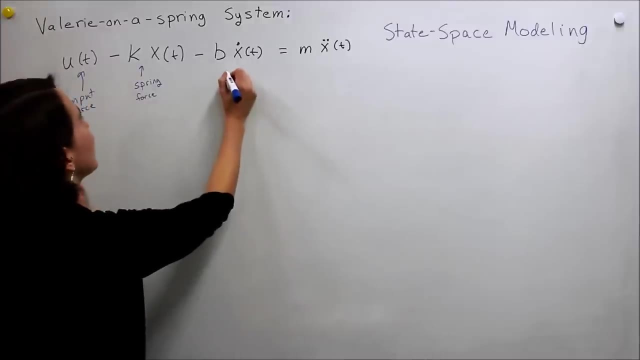 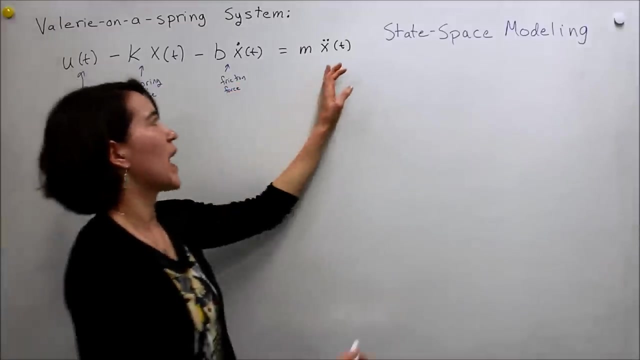 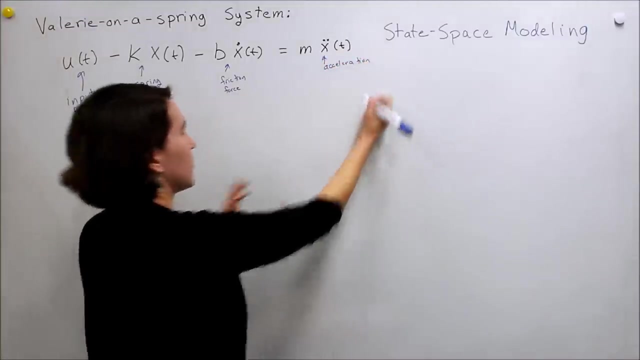 Valerie, This was a spring Force. Technically, this is right, the sum of the forces. And then this was friction. And then on the other side we had the mass times, the acceleration. OK, so now you remember kind of where this comes from, And we got it into this form and then we took the Laplace. 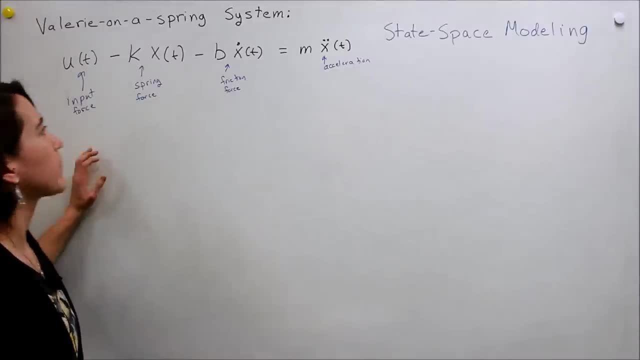 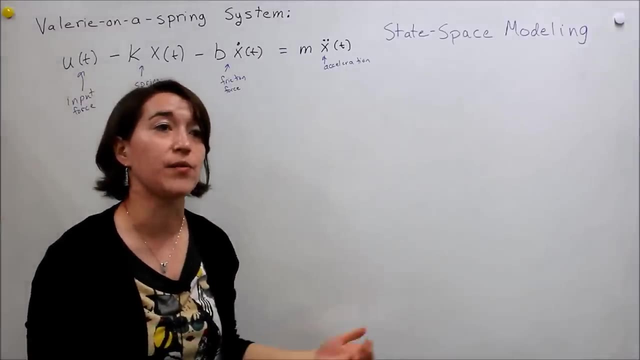 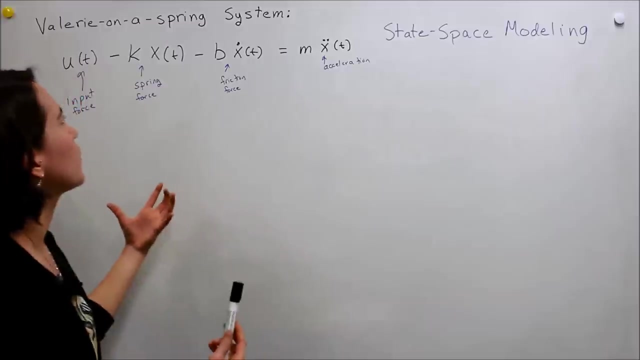 transform. But there's another step that we can do And we're going to use state space modeling to model this And later on we'll talk about how we can do various types of analysis on the system, But what we can do, so some people may get confused with. 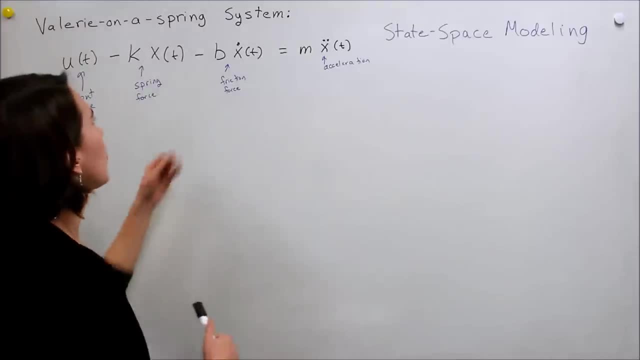 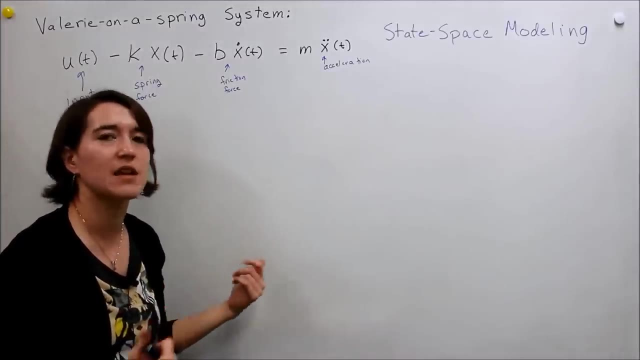 you know, you have x as one state and we chose that to be our output. But we also have x, dot, and that's the velocity right, So the velocity of Valerie as she's moving. So in some ways that's another state. So the idea of state space is that we assign states. 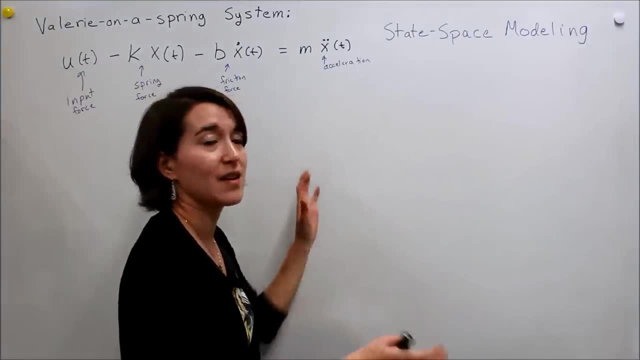 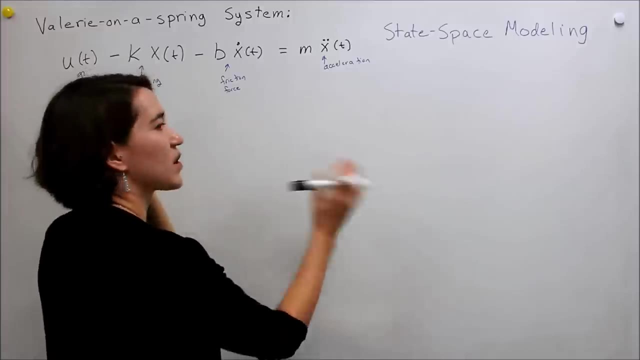 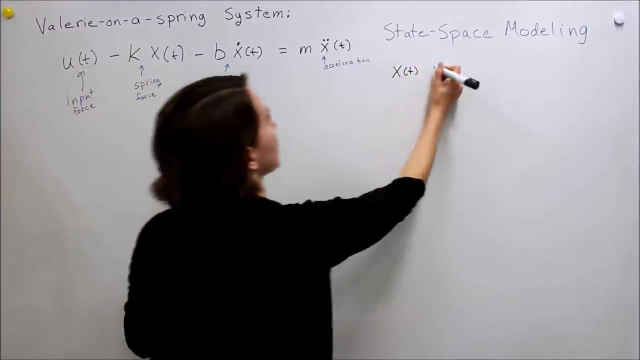 to each of these And we look at each of their dynamic equations separately. So what we can do is say we get confused with these derivatives and we want to just rename them. So we're going to say we're going to call x of t which we have here, We're just going to call that x one. 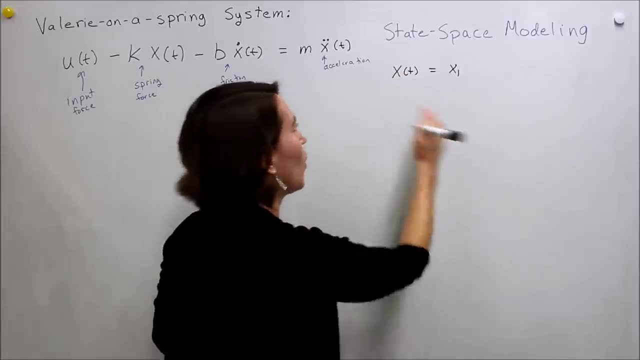 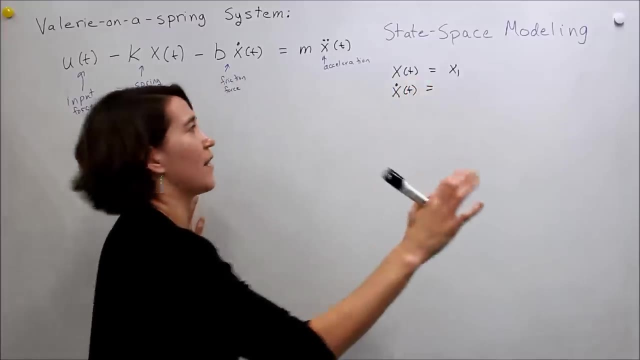 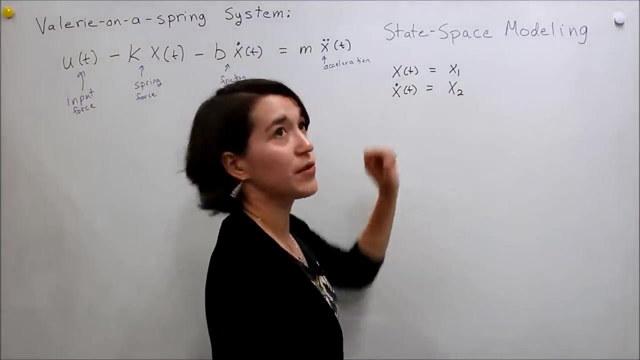 And then in this I'm going to drop the of t's, So hopefully this won't be too confusing. And then let's just say the velocity, which is x dot of t. we are just going to call that x two. Okay, And notice, there's actually a relation between x one and x two now, Because x one 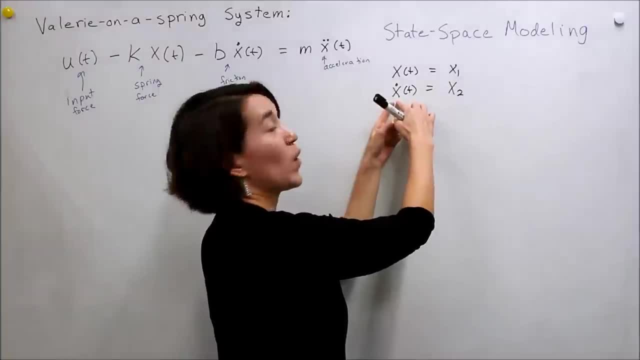 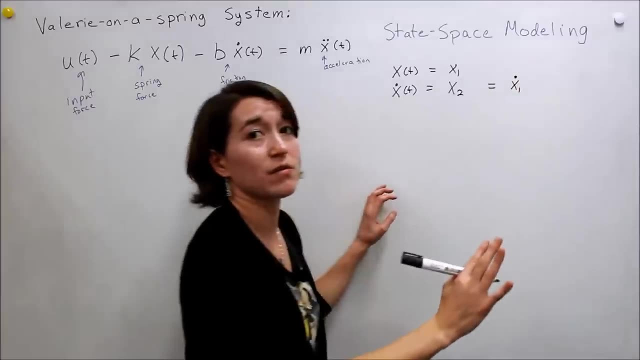 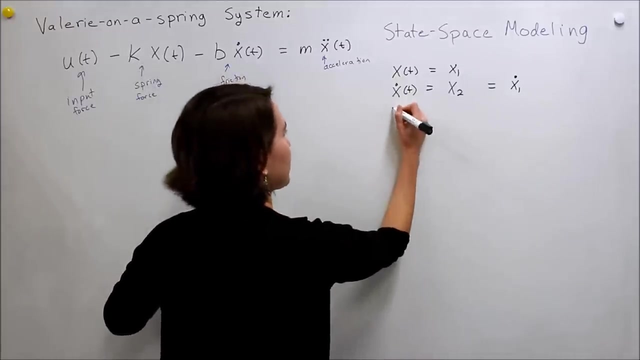 is x. the derivative of x one is x two. So we're just going to write this over here as kind of a side note: x one derivative is equal to x two. So we're adding some changes in variables here. We're for completeness, we're going to call u of t And then we're. 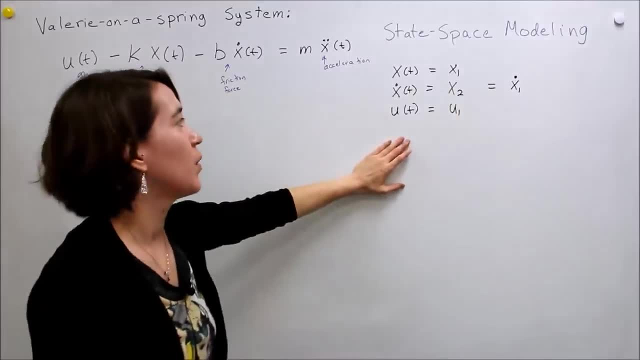 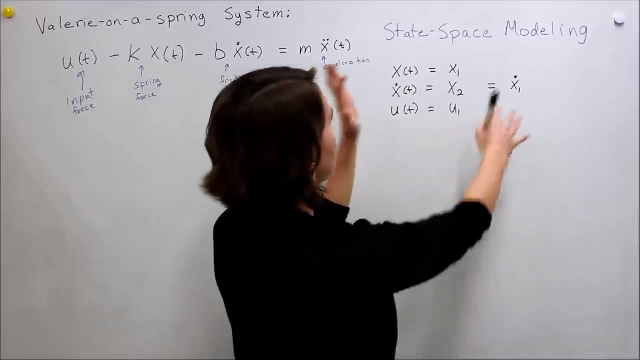 just going to call that u one. Here we only have one input, but we could actually model multiple inputs here, So for now we'll just call u u one. Okay, so we have some new equations here. We changed our variable names, So first of all, let's 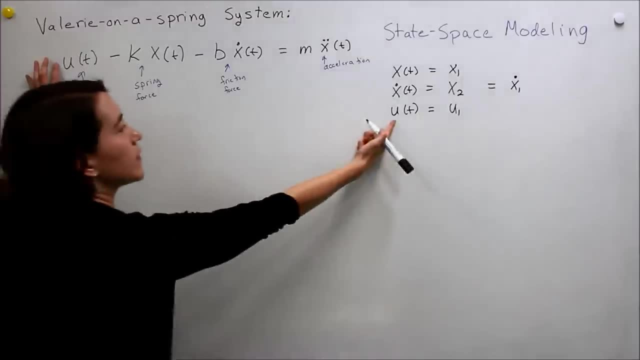 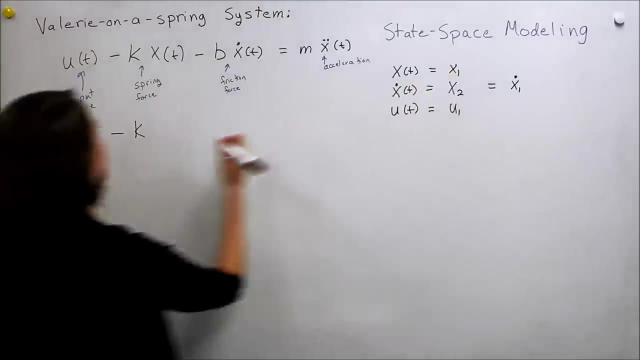 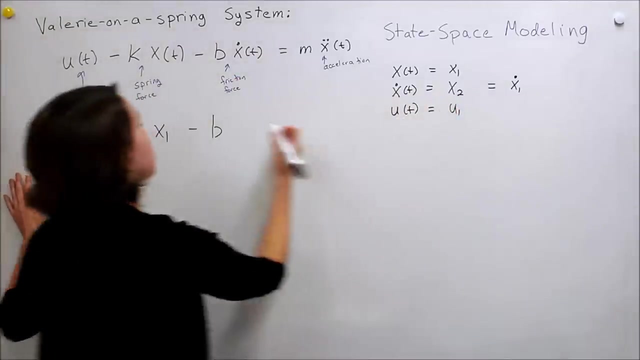 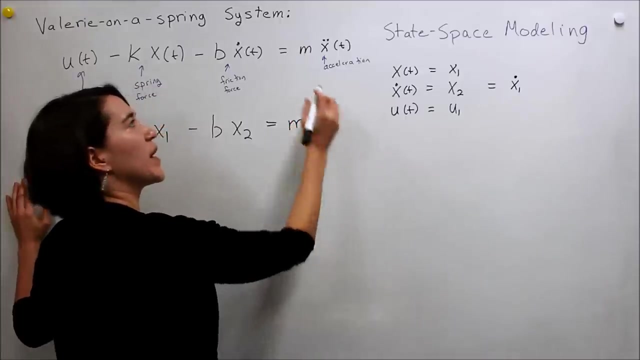 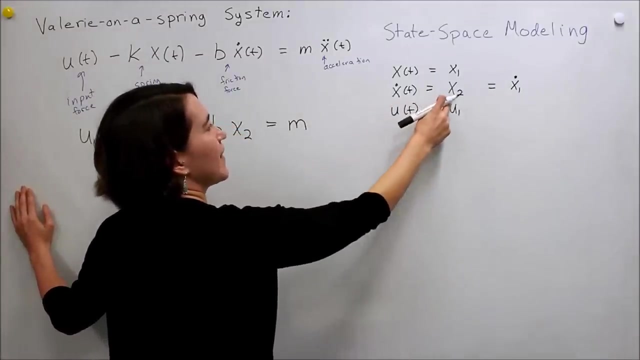 put that into this equation. okay, So u becomes u one, so we have u one here. minus k is our constant. still, X is now x one, b x dot is now x2, right x2, and then M, and we have our x double dot, which is actually the derivative. 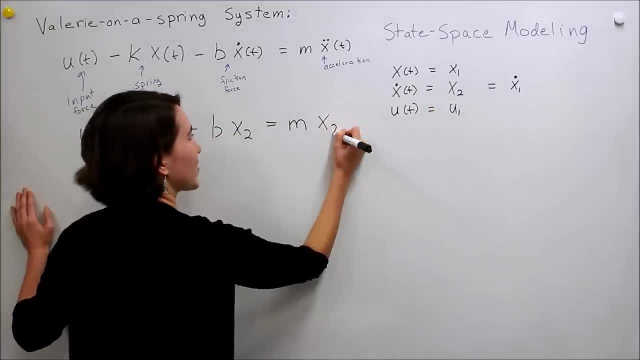 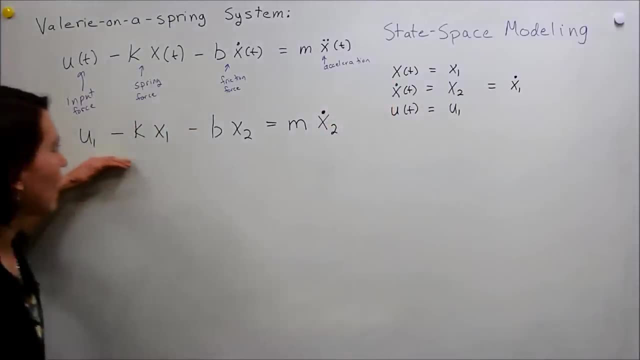 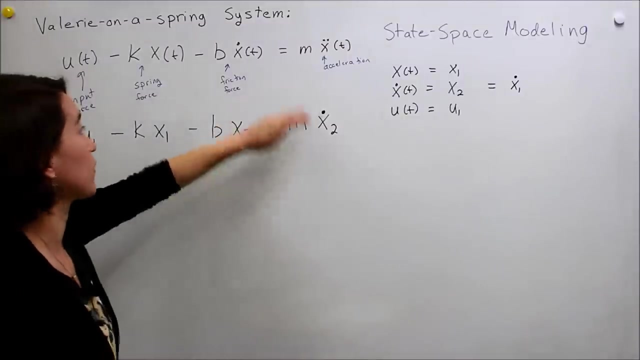 of x2, so x2, which is single dot. take another derivative and we get x2 dot. okay, so you're following me. so we have put everything in terms of our new equations and we have. we have one x2 dot, but only a first derivative here. okay, with this expression and what we can do here. now what? 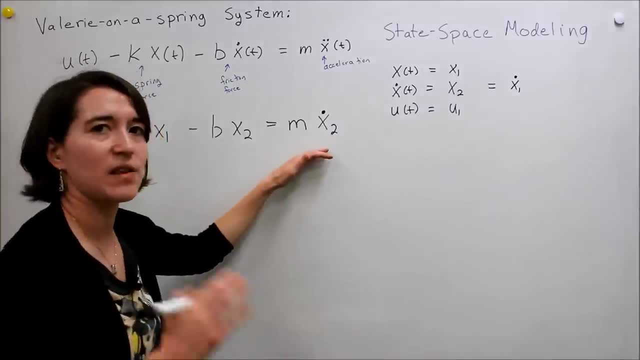 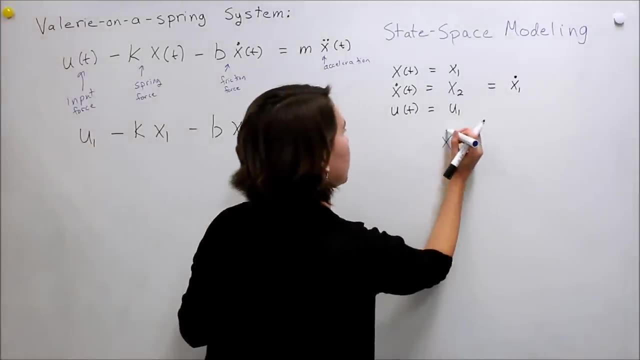 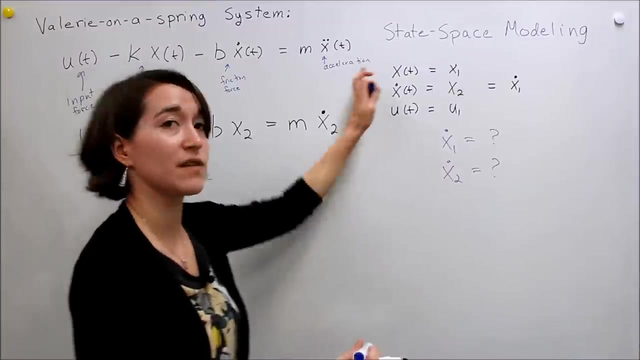 we want to do in state-based modeling is take each of the states and look at its dynamics. so really, what we want to do is find x1 dot is equal to something, x2 dot is equal to something. so you want to find the derivative of each of these. 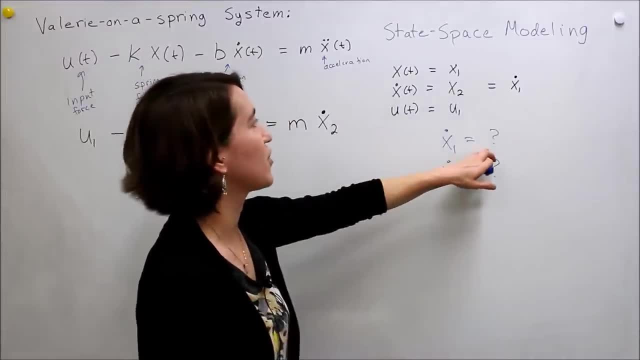 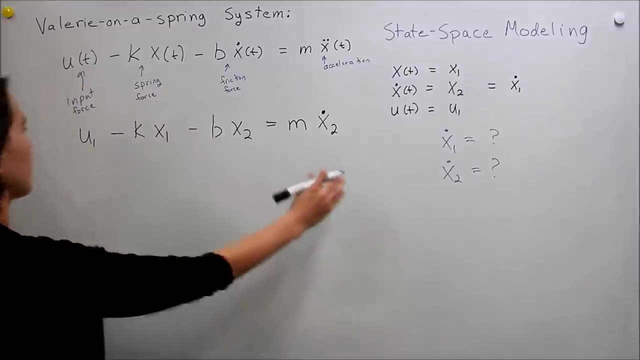 states as an independent equation and this function should be in terms of these other equations, these other terms here. okay, well, so let's, let's look at this. so let's try: X 1 dot. if we look at what we've written here, we see that X 1. 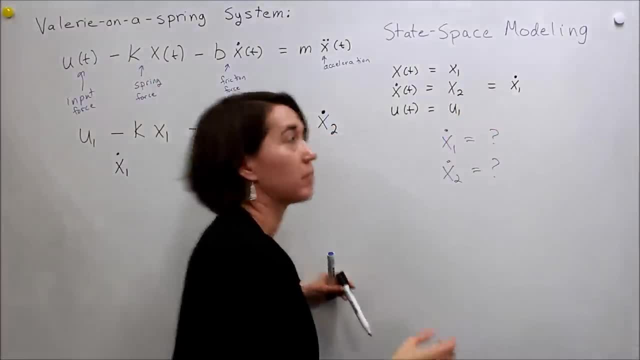 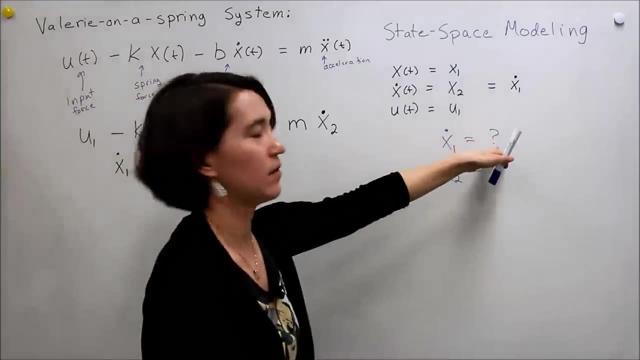 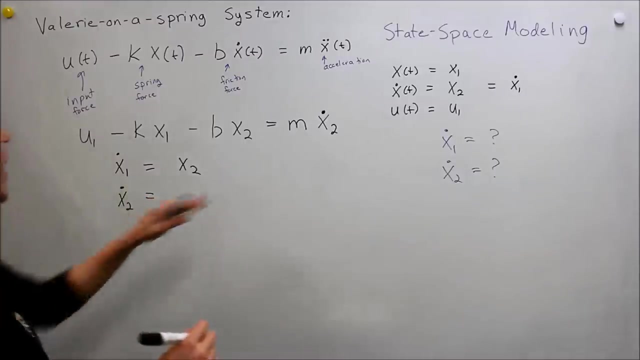 dot is equal to X 2, because that's how we defined it, so we can say: okay, well, that is equal to X 2. okay, so that's, we've found the answer to the side. now, what about X 2 dot? well, we have this equation right and we have our X 2 dot. 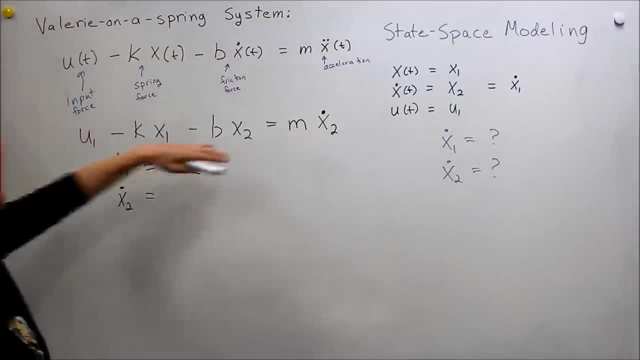 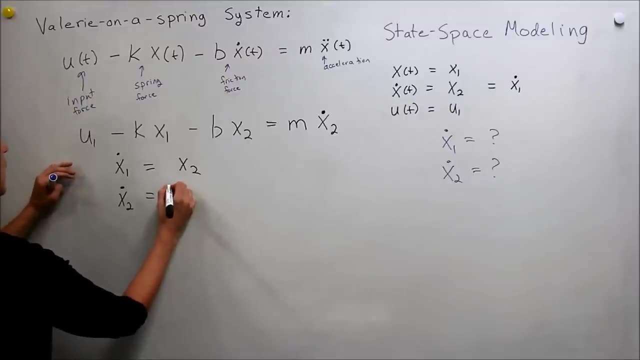 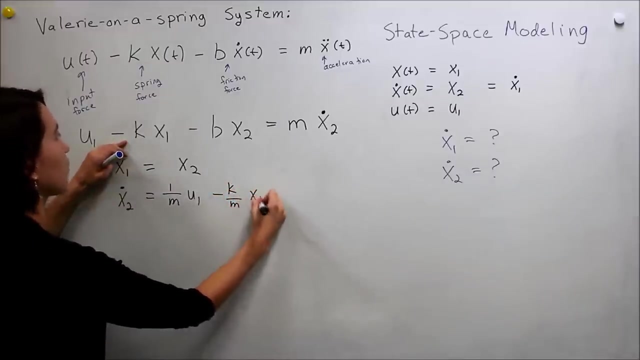 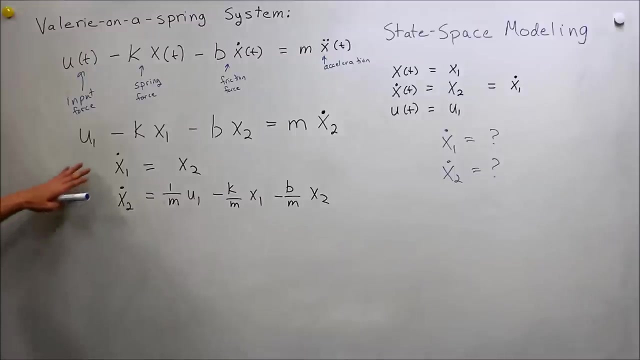 here. so if we want to write that independently, we can move this M over. divide the whole thing by 1 over M and we can get. so we'll do 1 over M, u1 minus K over M X 1, minus B over M X 2. alright, so we found an equation just by renaming our 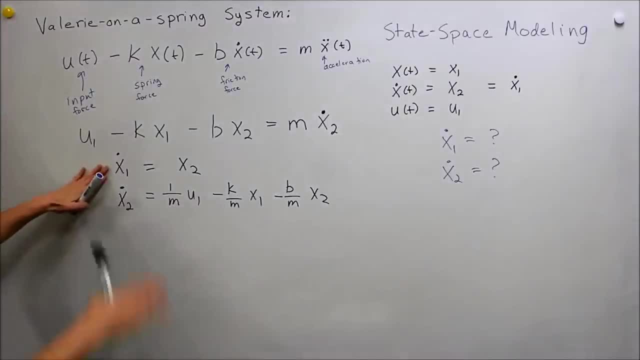 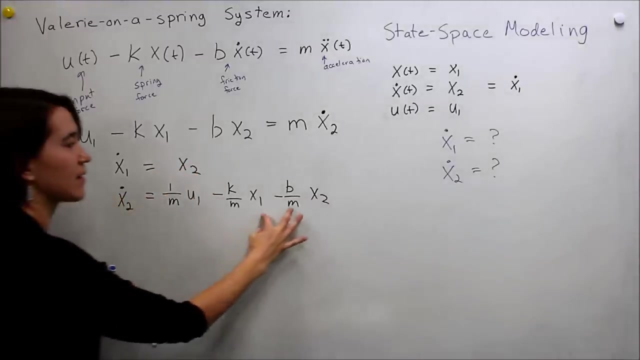 variables here and we have X 1 dot equal to something and X 2 dot equal to our other variables. what we can see by looking at this is that, well, X 1 depends on other states and X 2 depends on the other states and the input. 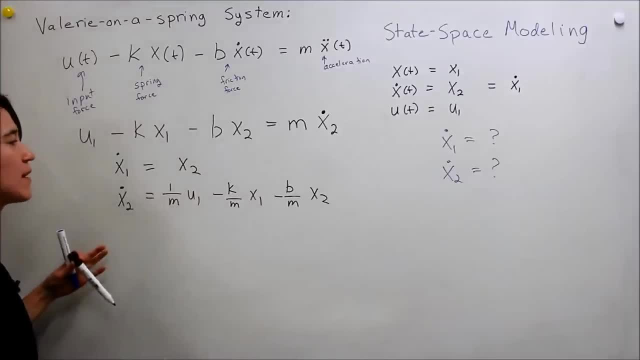 so if we want to break down our system, we can see, well, how does the system relate to itself- meaning X 1 and X 2, because those are states in the system- and how to each of these states relate to the input. so we're actually going to 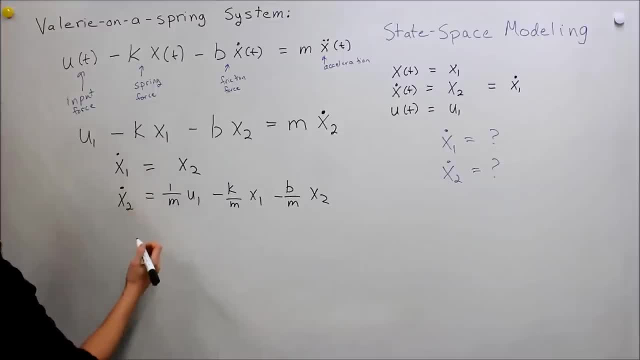 break apart our system a little bit. so well, we're gonna rewrite these and, yeah, we'll do this here. so X 1 dot is equal to. we can write it as we want to know how x1 relates to X 1, X 2 and u. that's right, and so all we need to do now is say: that X 1 X 2 exactly does differ from the previous equation, because that's a power of the operator that works on the BER Basharğ model. okay, so we just凧. Okay, now we're gonna go and write this down and you're gonna need some. 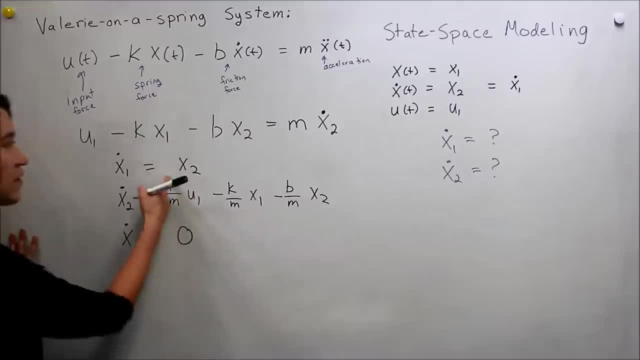 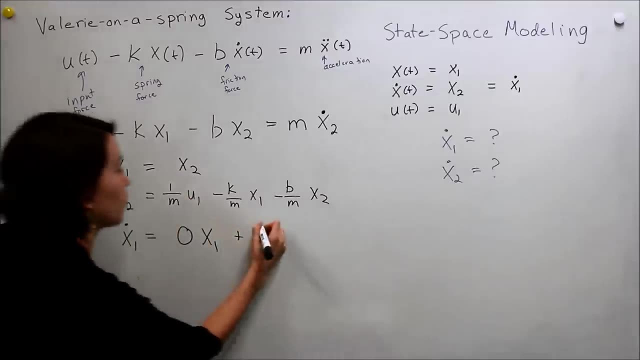 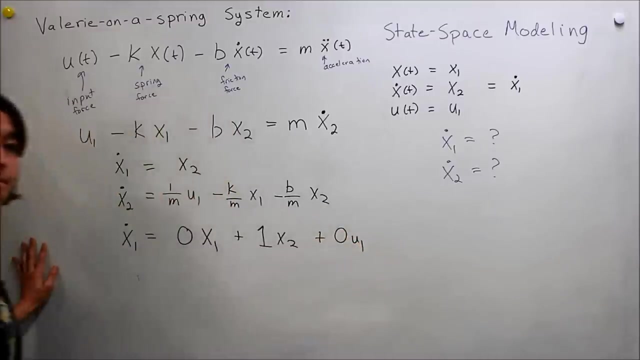 So let's write those all down. So it doesn't relate to itself. it doesn't relate to x1.. So 0 times x1.. It does relate to x2, so it's 1x2.. And this does not relate to the input, so 0u1.. 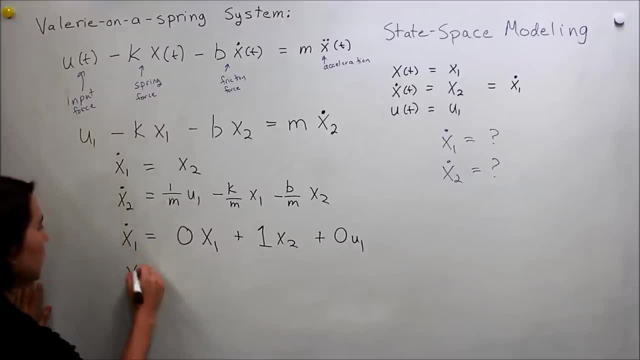 All right, so let's write the same thing here And here I'll put a little line. So we're looking at, we're changing these around a little bit, And OK, so what about x1?? So, oh, so this does relate to x1.. 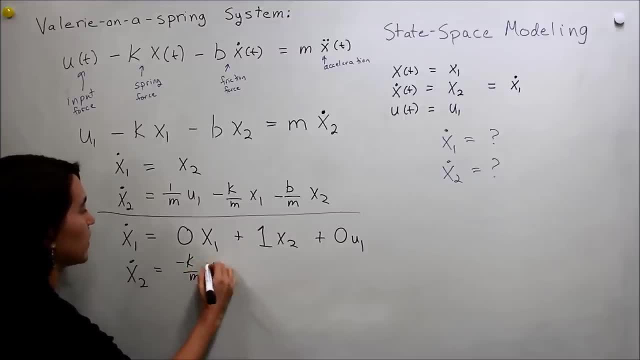 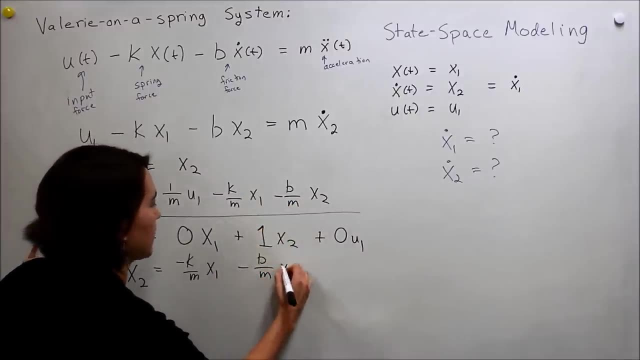 So we'll do negative k over m x1.. And what about x2?? Oh yep, here's something So negative b over m x2.. And does it relate to the input? Yes, by 1 over m. 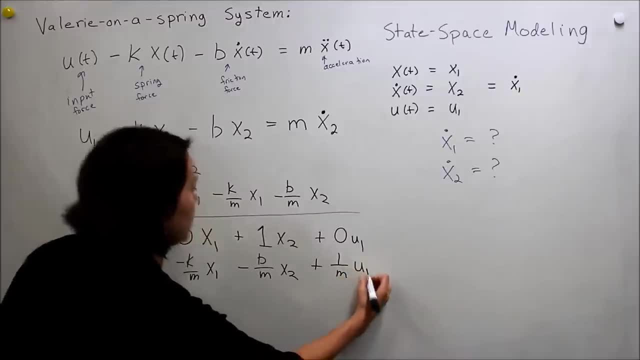 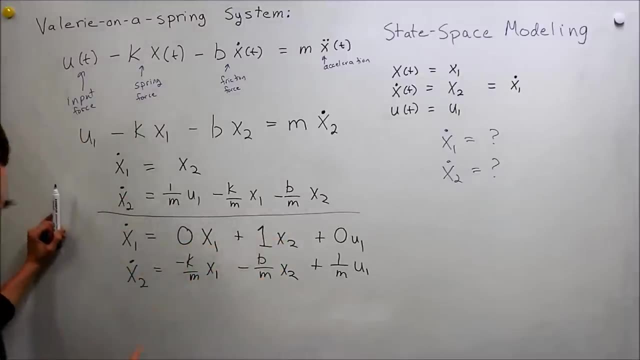 So 1 over mu. And what we can do here is: well, we have x1 here, x2's here. we can actually turn this into a matrix, So we can write this and we can make these vectors. So we're just kind of changing our notation here. 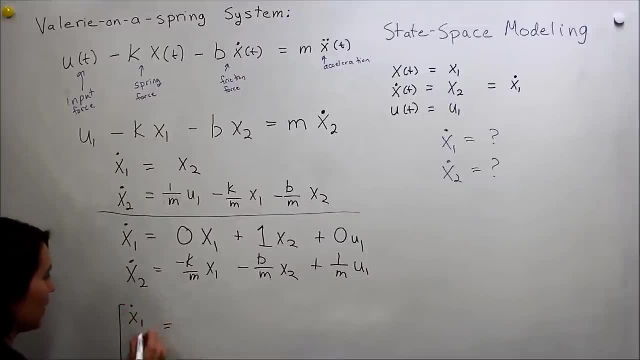 So it's x1 dot, x2 dot. use it as a vector, And then we are going to take the coefficients here and make them into a matrix. So we get 0, 1, negative k over m, negative b over m. 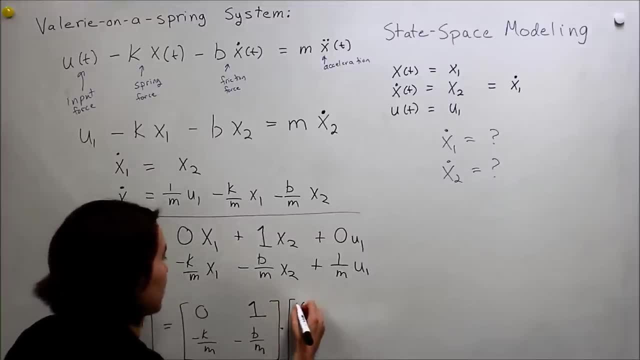 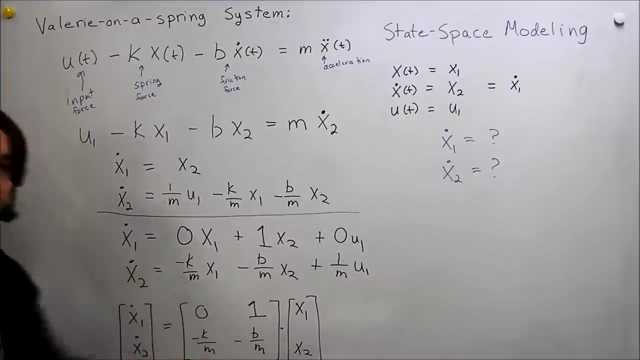 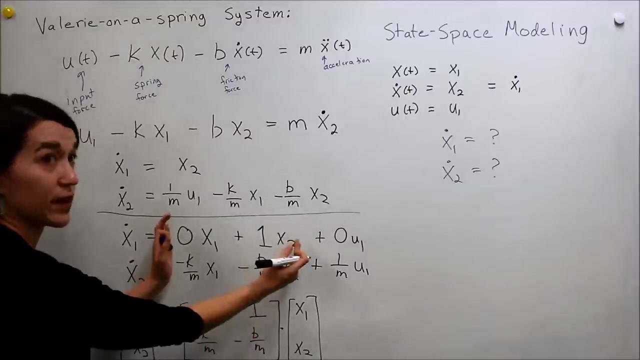 And then if we multiply this matrix by our vector, x1, x2, right in the same order. so first row will be x1, second row will be x2, then we have the same expression for this. So what about this last one? 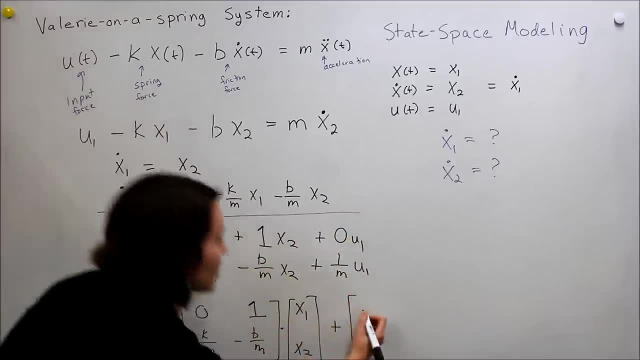 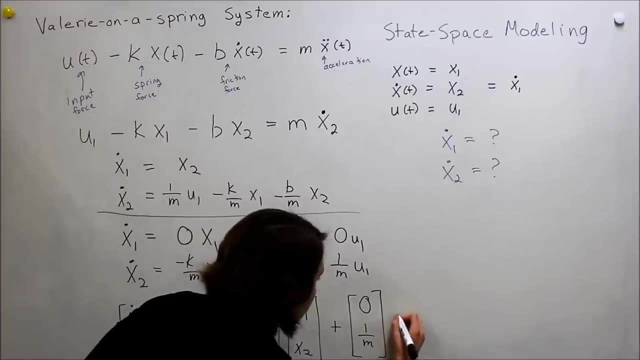 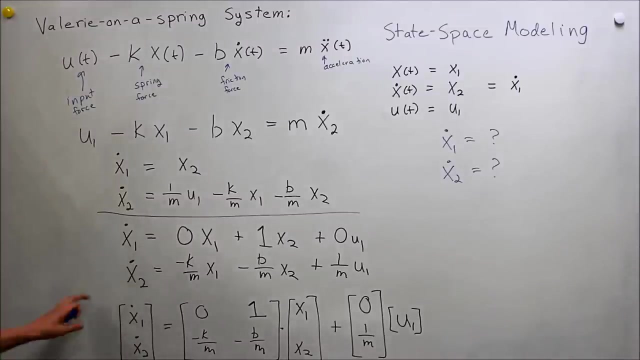 Well, we can do the same thing, Model this as a matrix. so 0, 1 over m, And then in this case there's only u1. So we'll do u1.. So we've actually modeled our system in using matrices. 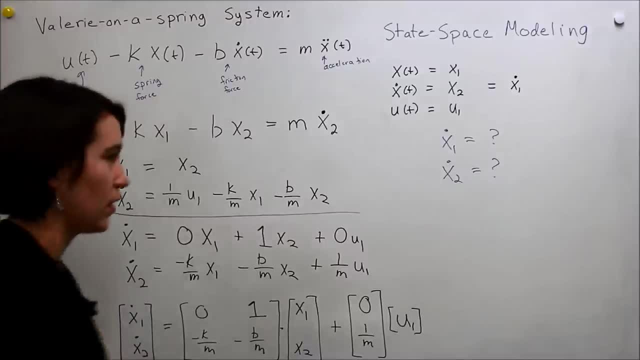 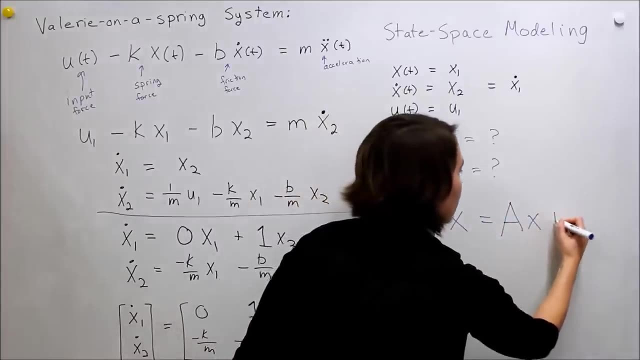 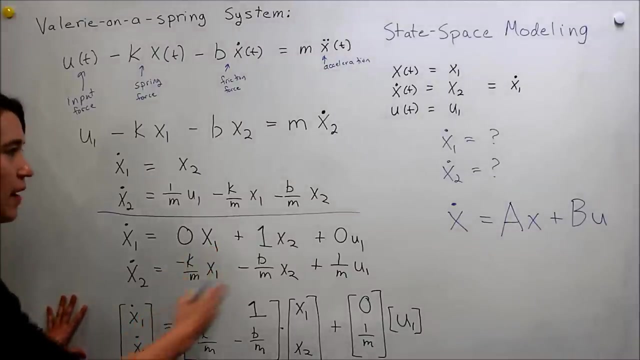 And this is a standard form that we can use for our system. The standard form that we use is: x equals ax plus bu, And what we've done essentially is x. here is the vector. So we have a vector x1, x2.. 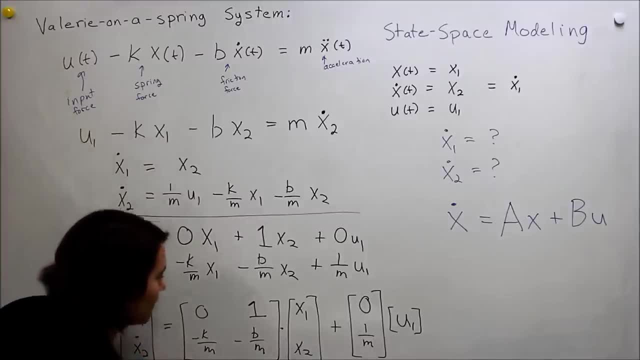 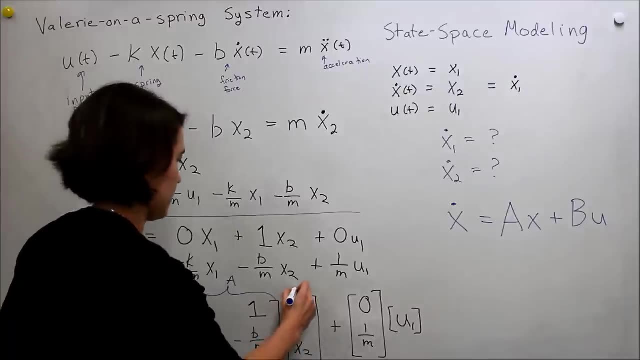 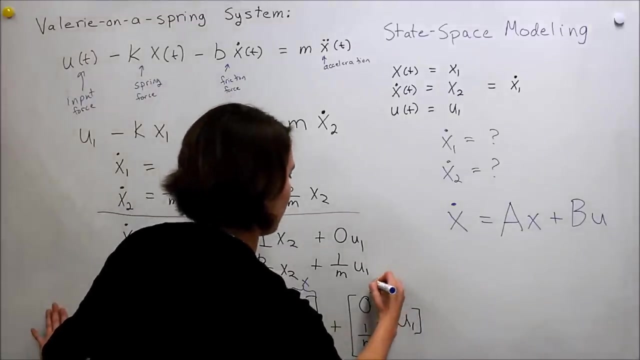 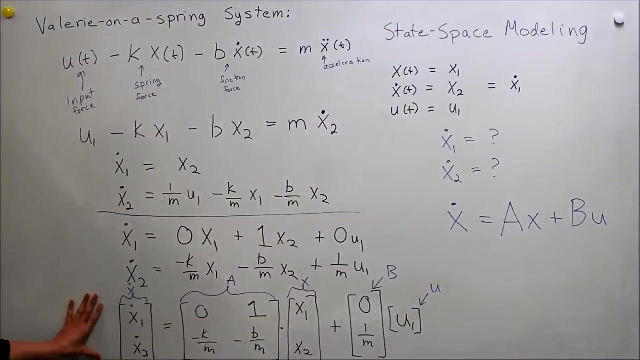 Those are states. That's what we call them. This is a. I'm going to put up here a. This is our x, This is our x dot And this is our b And u. So this is a standard form for modeling in state space. 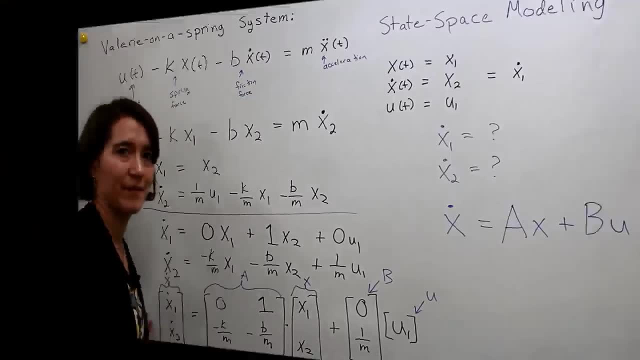 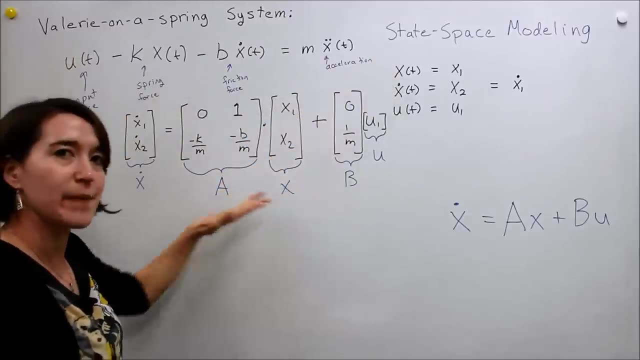 And then what we'll do is actually, you know, is maybe we'll save this And we'll talk about the output next. So we've modeled our Valeriana spring system from this original equation and we've put it into a state-space form. 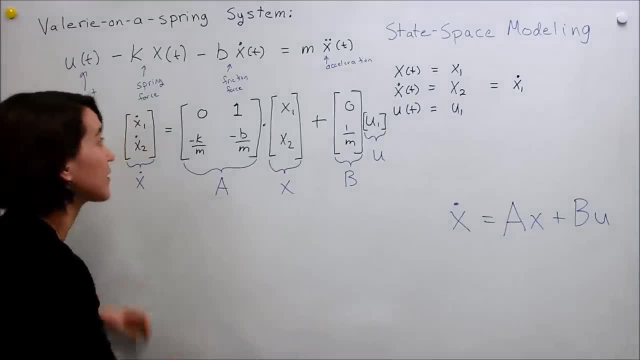 We're almost there. We need to look at the output now. So this is our system, but what is our output Before? we decided that x- the position of value- is our output, So in the standard controls language we write x as y. 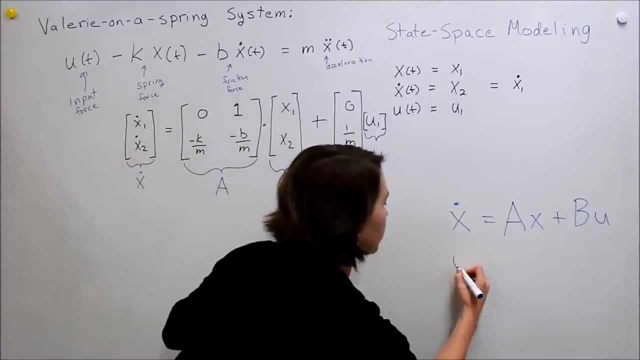 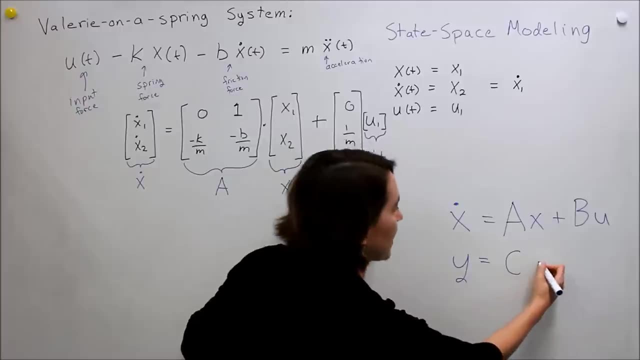 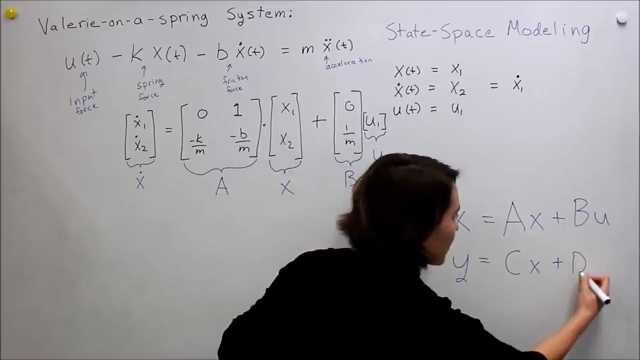 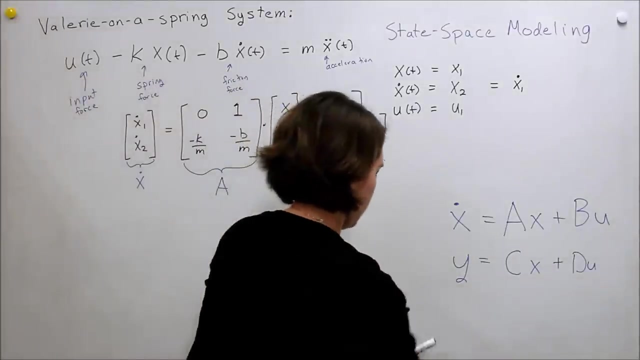 So we'll put it into a form where y is the output and it will depend on some matrix times, the x value. so the states: and it's possible that it might depend on the input value. But first let's just state that our output, in this case our output, y is going to be. 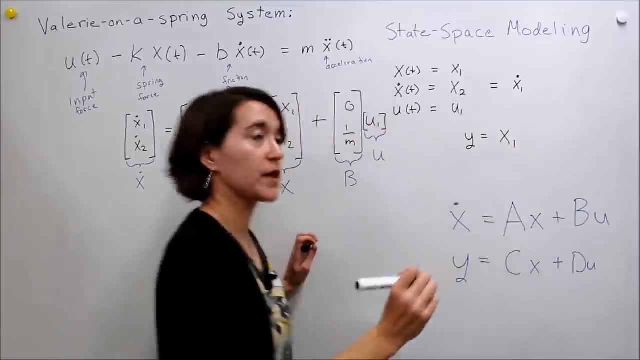 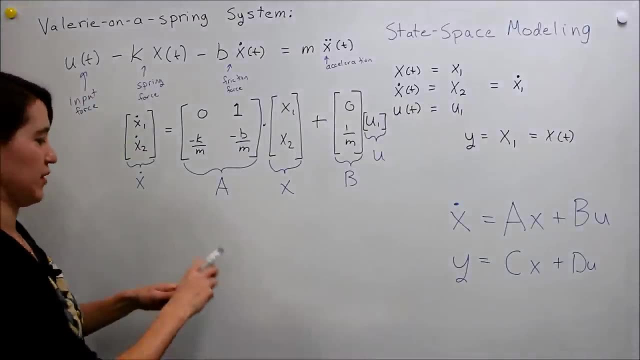 equal to Okay, Which is, if you remember, equal to x of t, Okay. So that's pretty simple. If we wanted to put this in a form, we have to see how y relates to x1 and x2 and to u. 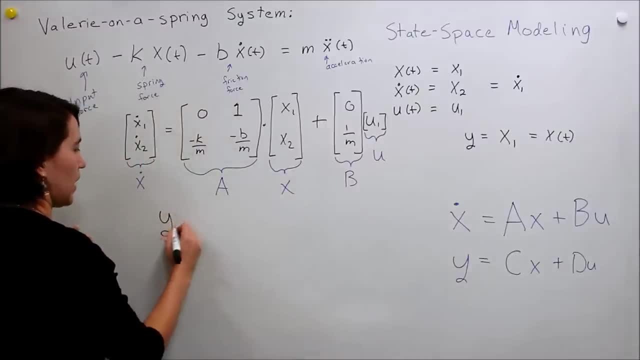 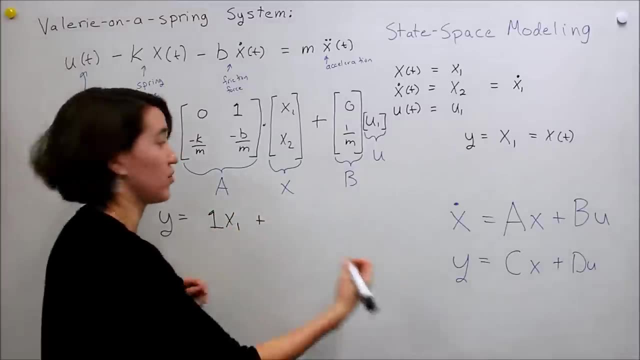 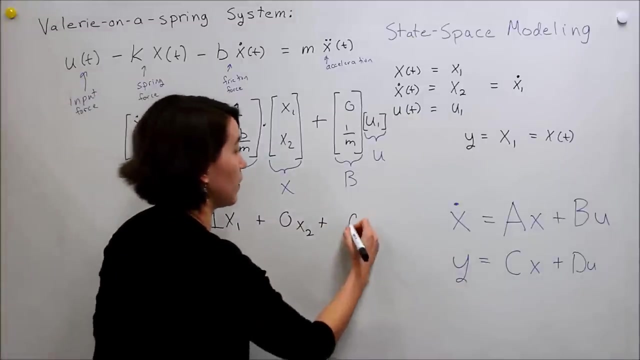 So if we wrote that out fully, we would get y equals to 1, x1, and does not relate to x2,, so 0x2.. And does not depend on u either, so it would be 0u1.. 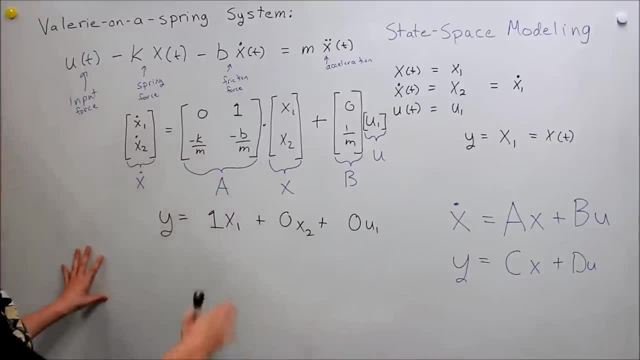 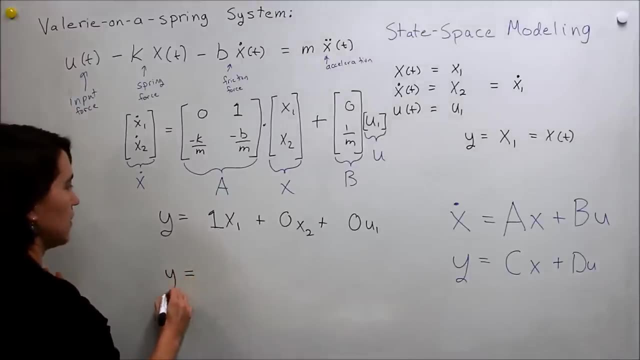 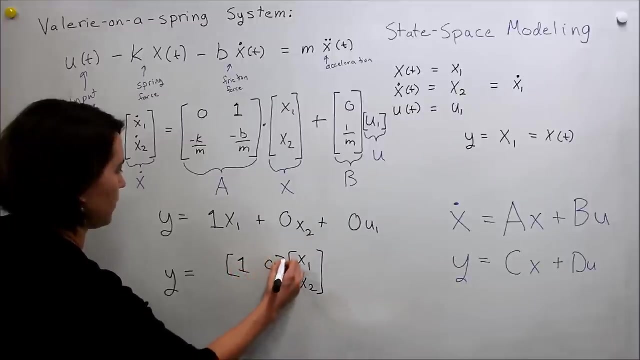 So if we wanted to rewrite that and put it in this form, well, we can put this into a matrix and simply write it as: So here's our x1, x2.. So Right, 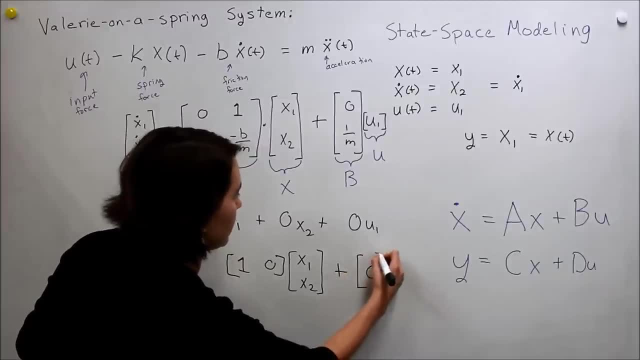 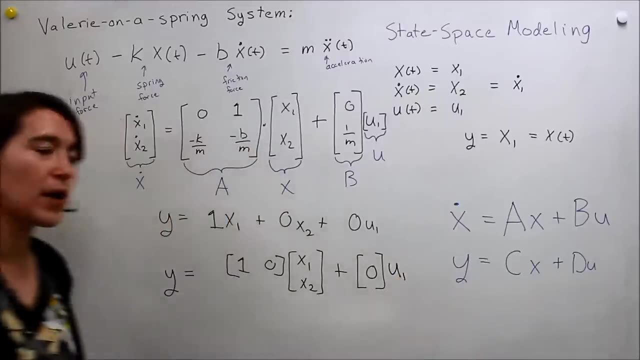 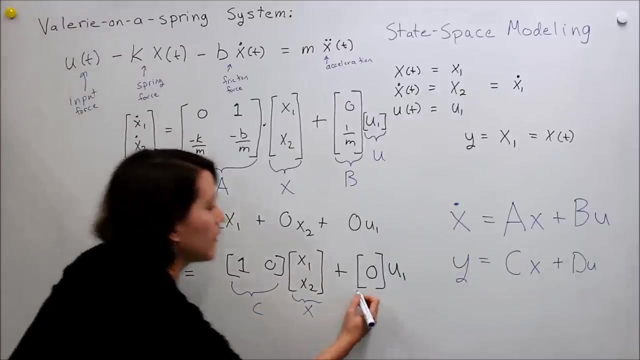 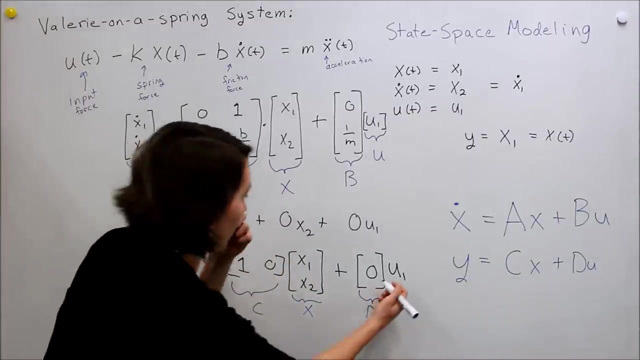 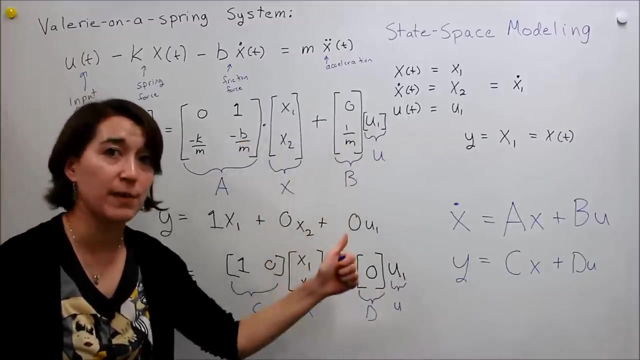 completeness. we're putting it there and then this again is U, and in this case we only have one input. but we could have a case where there's multiple inputs.